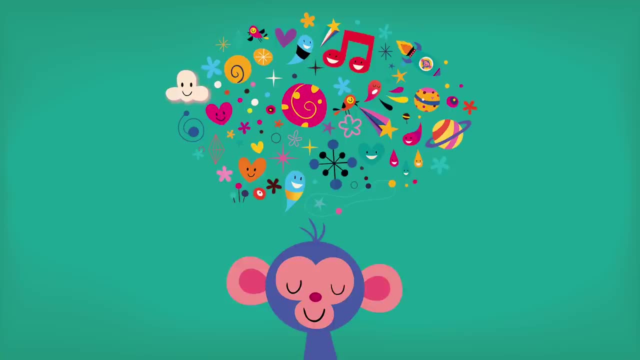 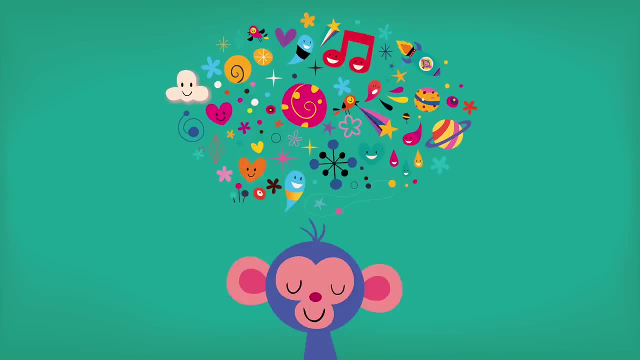 Feel them Really. feel the feelings that don't feel very nice. Just look at them, Not changing them. They are all allowed. Now see if you can notice your body. Imagine you are shining a torch all over the different areas, Having a good look. 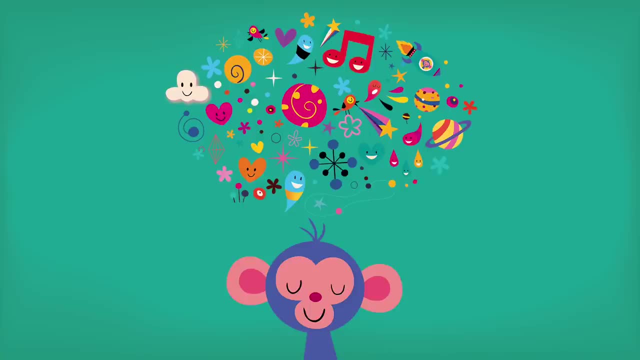 Is there anywhere in particular that you can spot? Can you notice any tightness or holding? No need to change it, just look at it. Now you are going to be a zen ninja and use laser sharp focus First. feel your breathing, your tummy lifting and lowering with each breath. 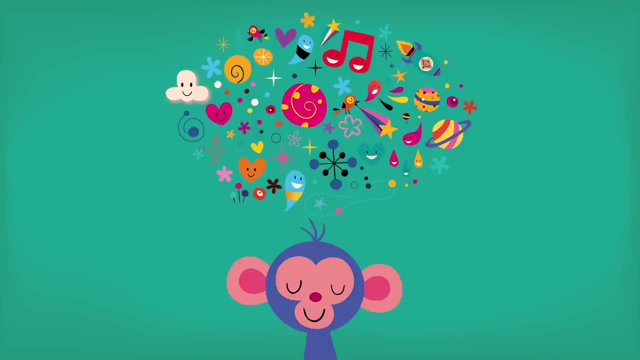 Keep your ninja laser on your breathing, Feel it coming in and going out each and every breath, See it, watch it, follow it. If your brain decides to wander back to those thoughts, spot it, like all zen ninja warriors do, and come back to your focus. 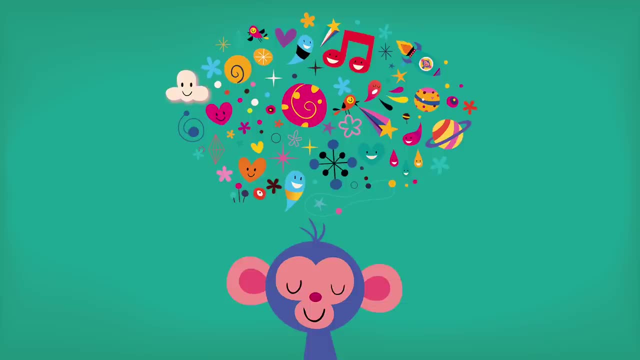 You're breathing in and out, In and out. Well done, You're doing a great job. See if you can imagine that your breath has made a big warm sunshine light up inside you, right in your middle. See if you can make the warm sunshine light up inside you, right in your middle. 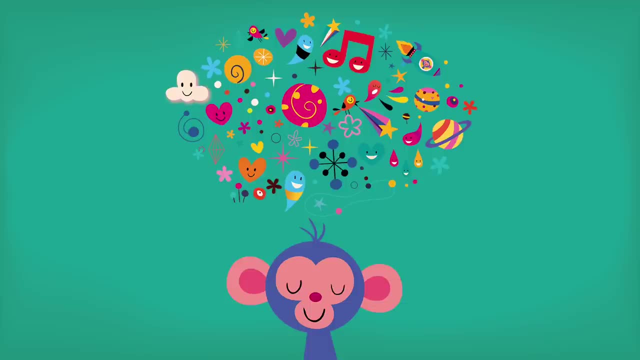 The warmth spread through your whole body. Like you are sending the sunshine down your arms, to your fingertips, down your legs to your toes, up into your head and around your face. Like you are filling yourself up with goodness. Now see if you can beam that warmth and sunshine further out.